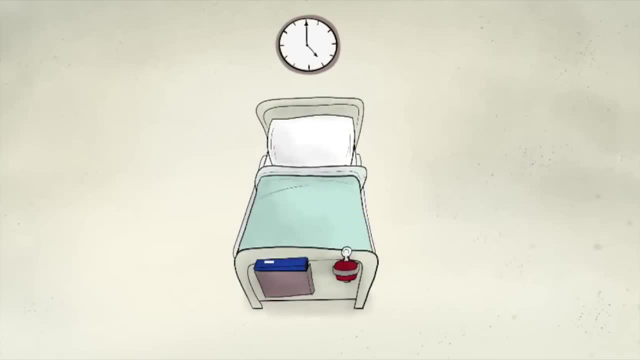 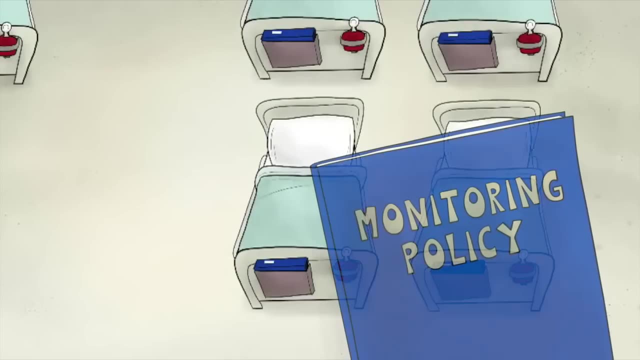 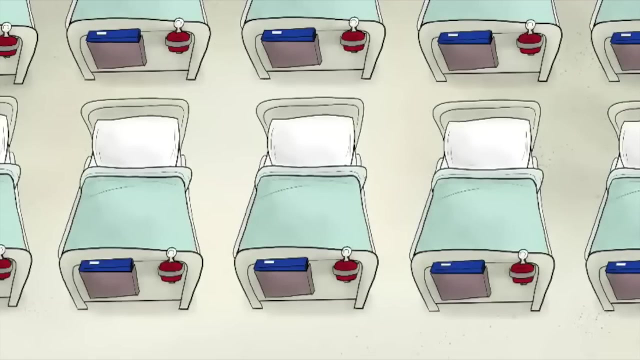 there are time pressures and the system isn't designed to make it easy to do the right thing. For instance, a patient may be unwell and the policy says they should have their observations done every hour. However, there are a lot of unwell patients on the ward. all the monitors that the nurses used to 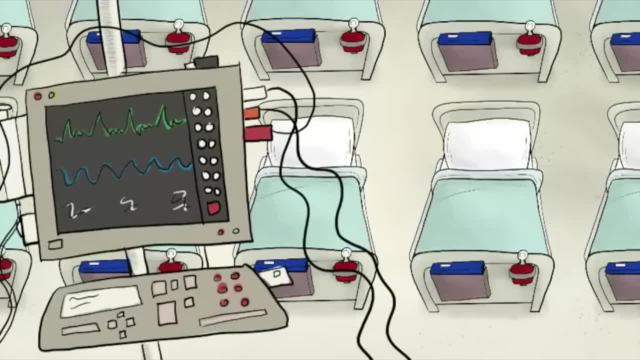 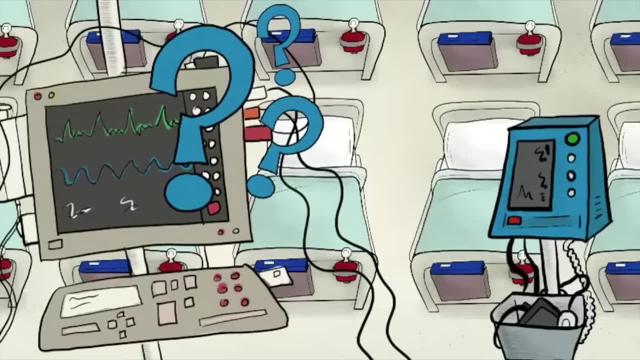 using are currently being used on other patients. There is another monitor available, but because this is different to the rest, the nurse is unsure how to use it correctly. Rather than try to use a piece of equipment that she is not familiar with, she waits until a different monitor becomes free. 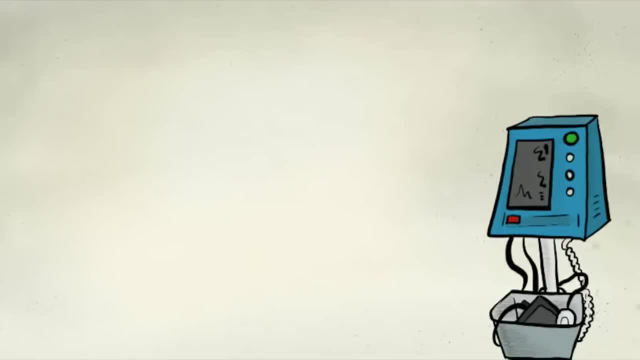 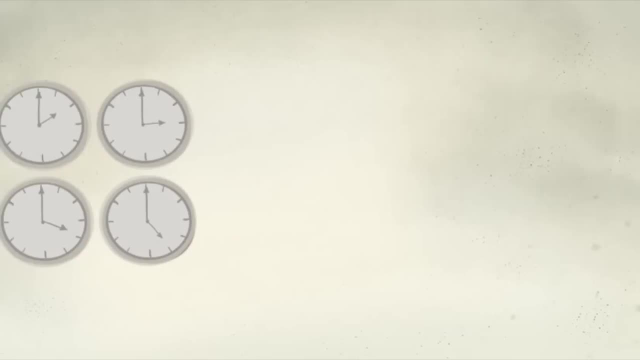 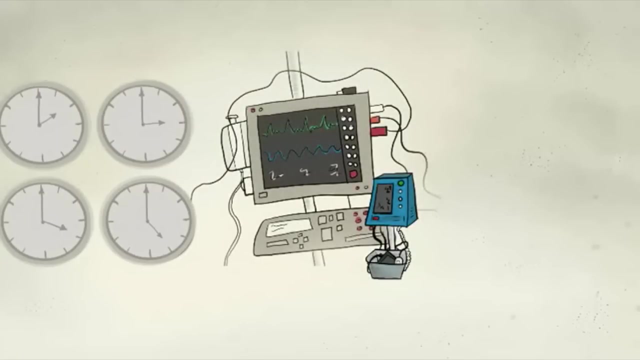 In the meantime, the patient deteriorates and this goes unnoticed In this situation. the nurse knew that the patient needed frequent monitoring and observations, but did not provide them. The reason she did not provide them was not because she didn't know what to do, but because the equipment 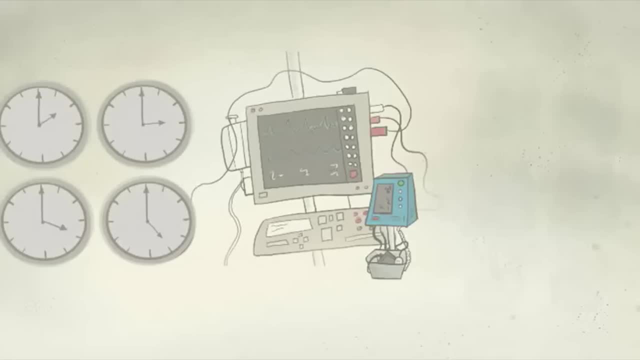 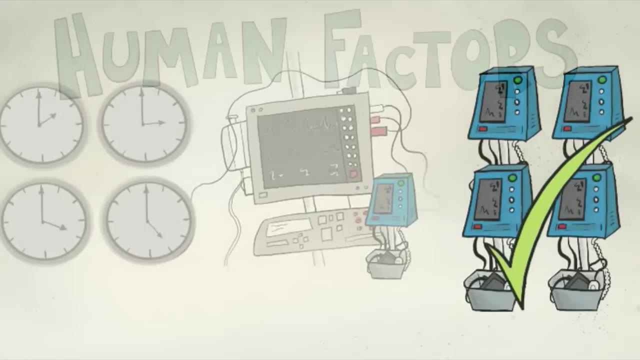 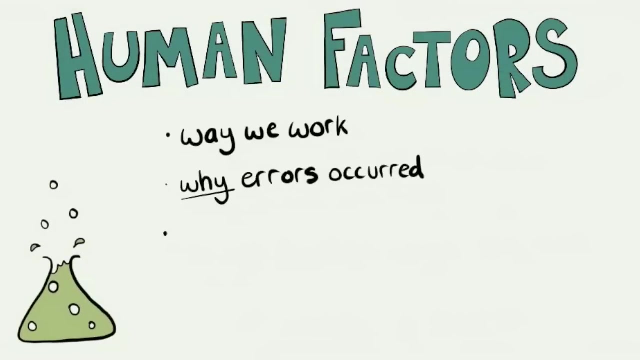 she was asked to use was different to all other equipment. This is an example of where having standardized equipment would have made it easier to do the right thing. The science of human factors can also help us investigate the way we work, find out why errors occurred and help design better. 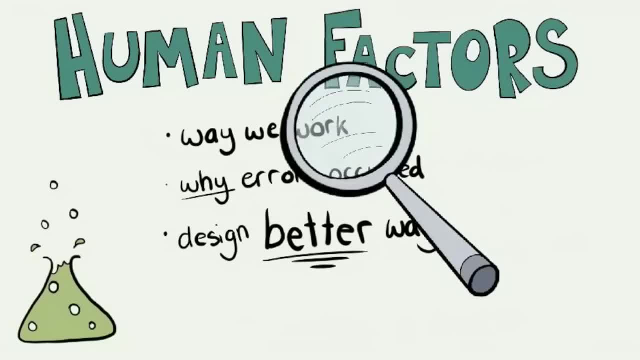 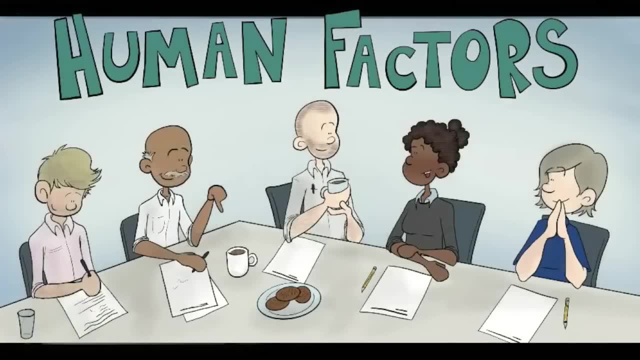 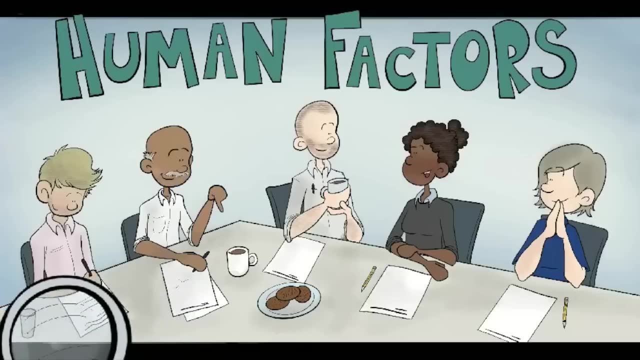 ways of working. The aim is not to be critical, but to gain a better understanding of exactly what makes their life difficult and what makes their life easy. Human factors awareness helps us prevent errors and helps us understand why mistakes occurred. This doesn't just mean when things go wrong, but also: 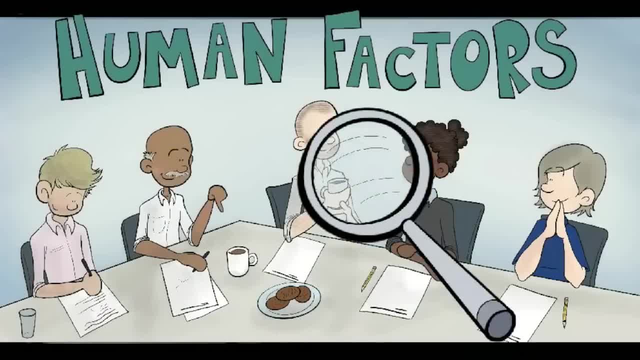 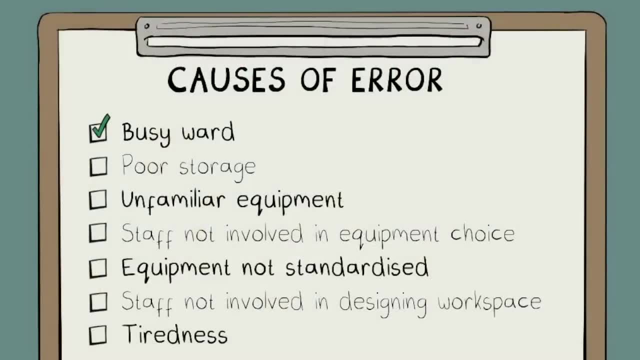 near misses as well. However, it only helps us if we are really honest in our investigations and acknowledge the real reasons why things go wrong. In doing so, we can understand why things go wrong. In doing this, we need to look beyond what happened when things go wrong. 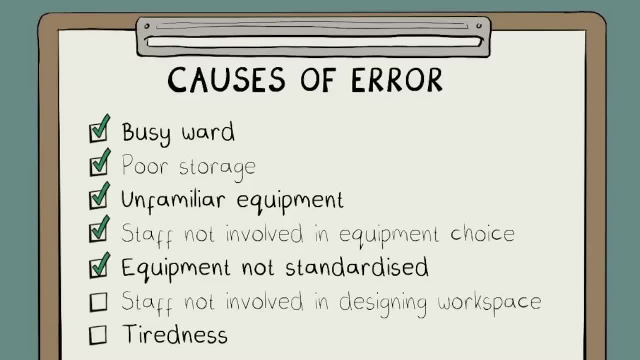 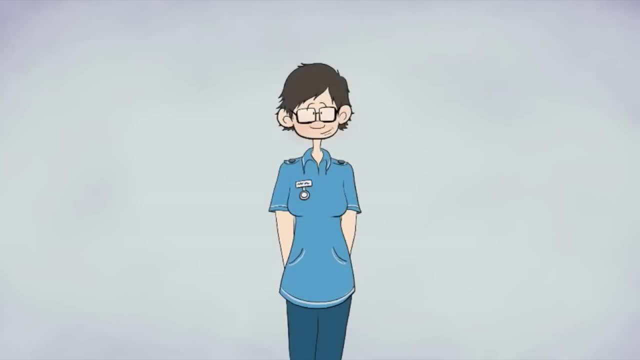 We need to go all the way back through the system and look at decisions made across the organisation that contributed to the error. This may include decisions made about planning and procurement of equipment. When investigating errors, human factors can help provide a better explanation of why the error occurred. 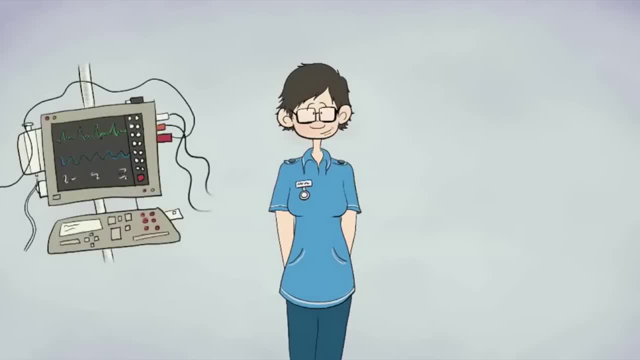 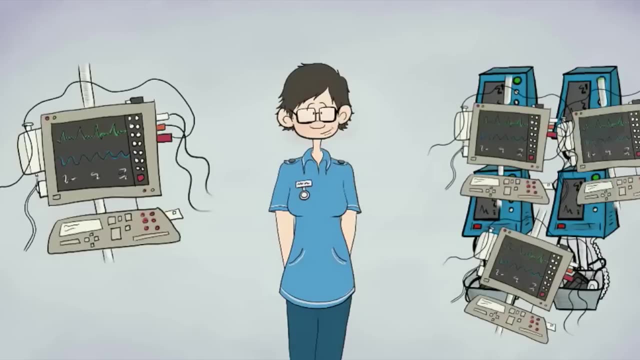 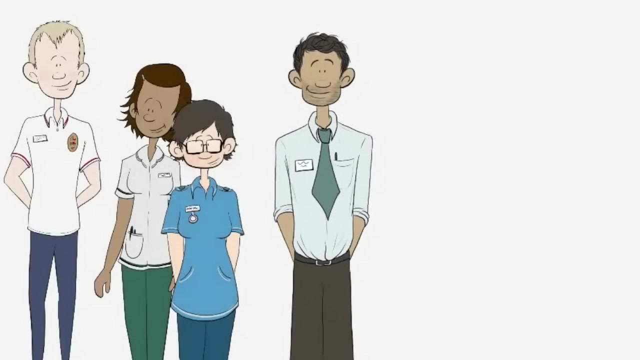 In the example of the nurse and the monitors. it would be inappropriate to just blame the nurse, because part of the cause of the error was down to equipment design and lack of standardization across the organization. we can't do this on our own. it is important that we all play a part in